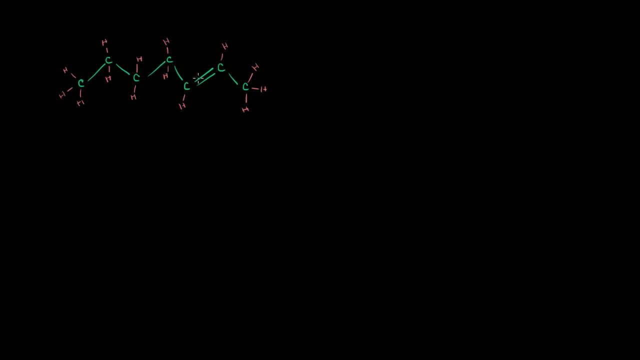 Because there's actually different ways that you can arrange it. because these double bonds are, you can imagine they're more rigid. You can't rotate around them as much. But don't think about that too much right now. Let's just try to name these things. 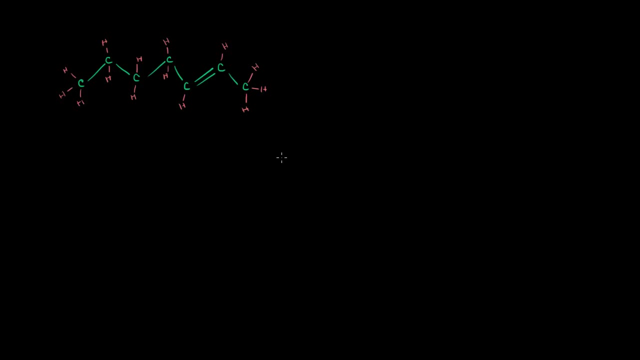 So, like we always do, let's try to find the longest chain of carbons. And there's only one chain of carbons here. There's one, two, three, four, five, six, seven carbons in that chain. So we're going to be dealing with hept. 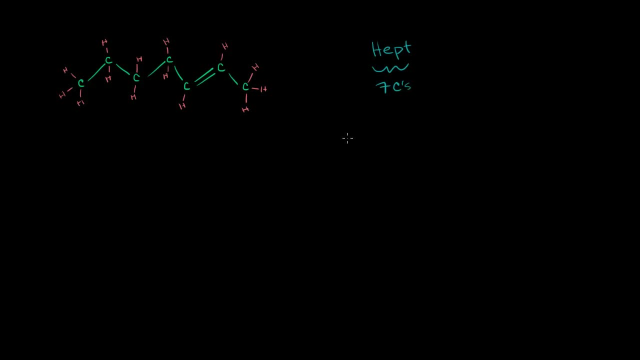 That is seven carbons, But it's not going to be in heptane. Heptane would mean that we have all single bonds Here. we have a double bond. So this is going to be an alkene. So this tells us right here that we're dealing with an. 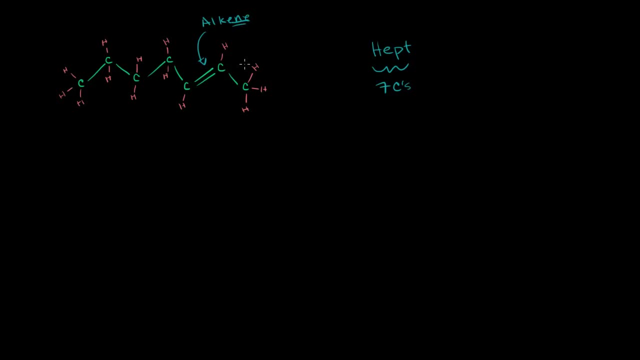 alkene, not an alkane. If you have a double bond, it's an alkene, Triple bond- alkyne. We'll talk about that in future videos. So this is hept and we'll put an ene here. 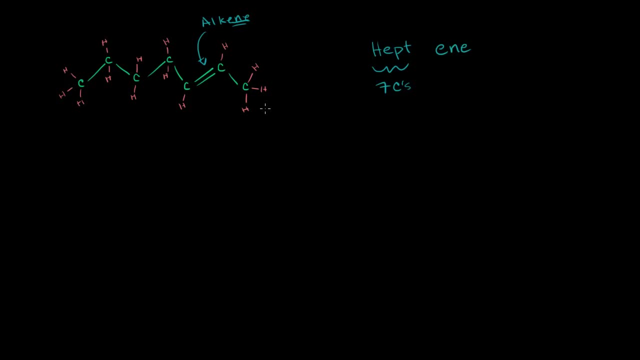 We'll put an ene here. But we haven't specified where the double bond is and we haven't numbered our carbons. So when you see an alkene like this, you start numbering closest to the double bond, just like as if it was an. 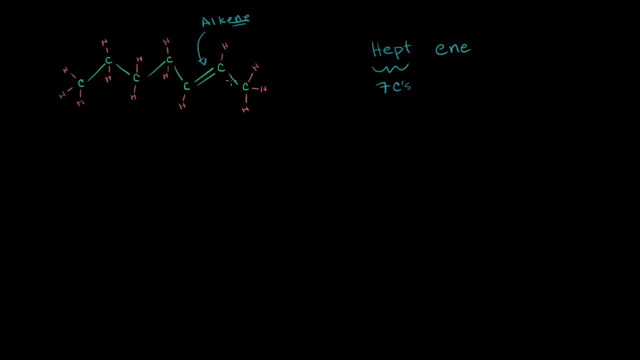 alkyl group, as if it was a side chain of carbons. So this side is closest to the double bond. So let's start numbering there. One, two, three, four, five, six, seven. The double bond is between the two. 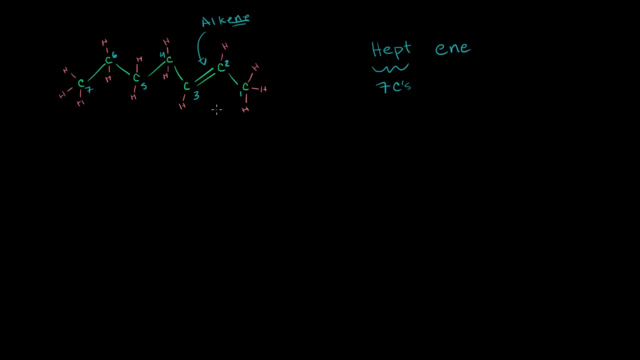 between 2 and 3.. And to specify its location, you start at the lowest of these numbers. So this double bond is at 2.. So this is actually hept dash 2-ene. So this tells us that we have a 7-carbon chain that has a 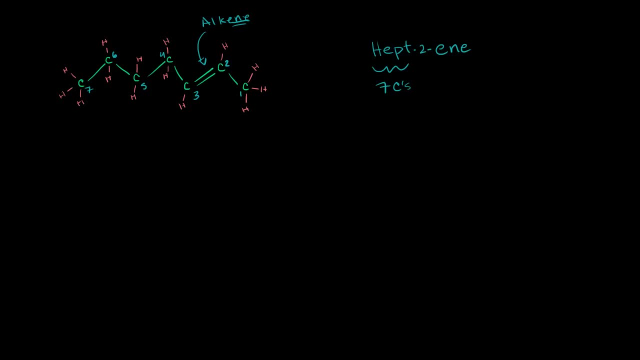 double bond starting. The ene tells us a double bond. Let me write that down. So this double bond right there, that's what the ene tells us. Double bond between two carbons. It's an alkene And the double bond starts. if you start at this point, the 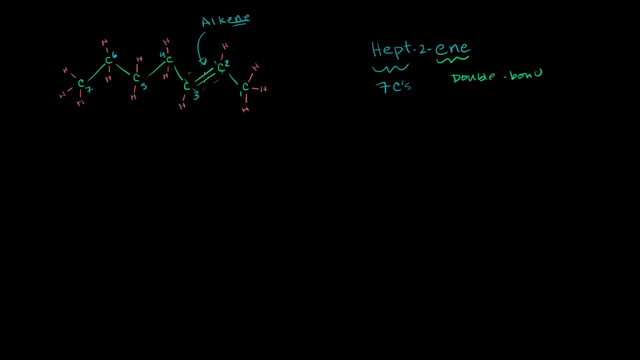 double bond starts at number 2 carbon and then it will go to the number 3 carbon. Now you might be asking: well, what if I had more than one double bond here? So let me draw a quick example of that. So let's say I have something like 1,, 2,, 3,, 4,, 5,, 6,, 7.. 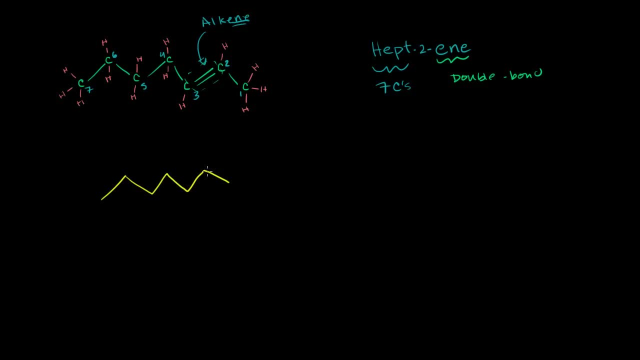 So this is the same molecule again: 1,, 2,, 3,, 4,, 5,, 6, 7.. The way we drew it up here it would look something like this: What if I had another double bond sitting right here? 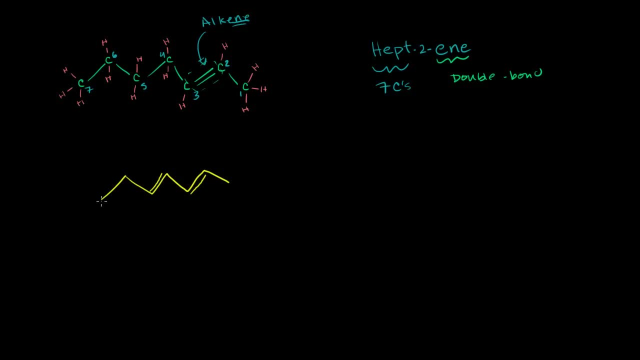 How would we specify this? Well, once again, we have 7 carbons: 1,, 2,, 3, 4,, 5, 6, 7.. So we're still going to have a hept here. 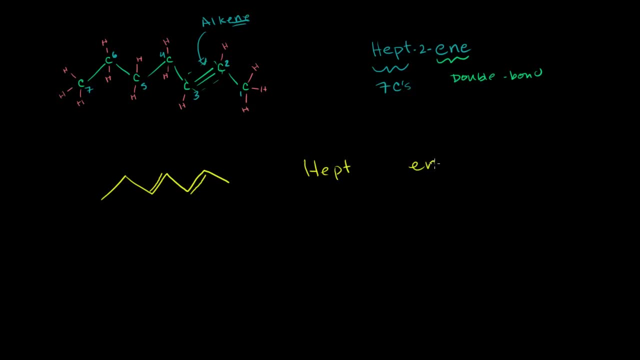 And it's still going to be an alkene. So we put our ene here. But we start numbering it once again closest to the closest double bond, So 1, 2,, 3, 4,, 5,, 6,, 7.. 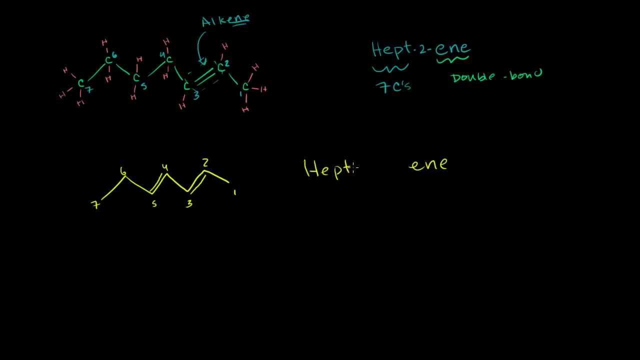 But now we have a double bond starting at 2 to 3.. So it would be hept 2.. And we also have another double bond starting from 4 and going to 5. So hept 2, 4-ene. 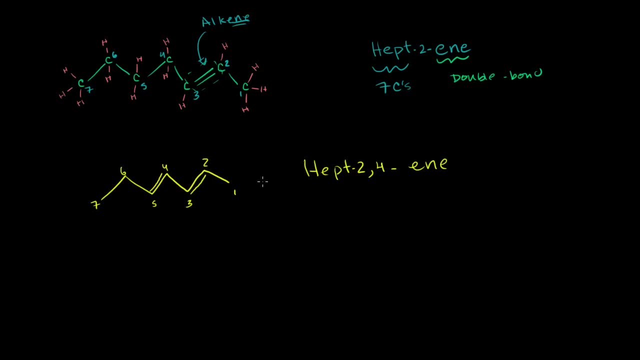 That's what this molecule right there is Now. sometimes this is the, I guess, proper naming, But just so you're familiar with it, if you ever see it. sometimes someone would write hept 2-ene. They'll write that as 2-heptene. 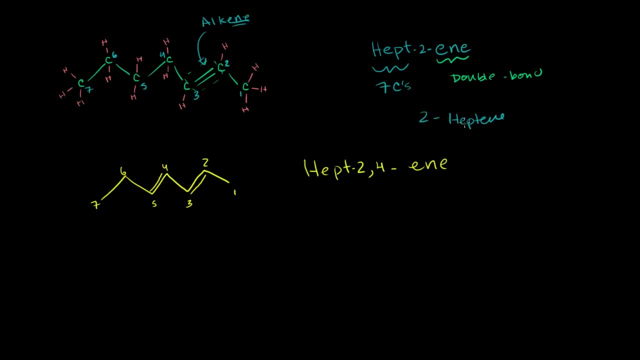 Probably because it's easier to say 2-heptene, And from this you would be able to draw this thing over here. So it's giving you the same amount of information And similarly over here they might say 2, 4-heptene. 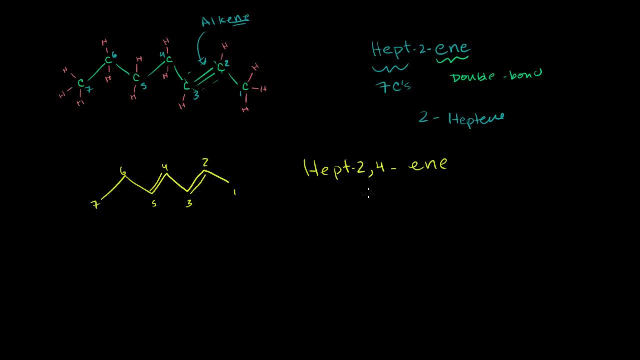 But this is the correct way to write it. It lets you know that the 2 and the 4 apply to the ene, which you know applies to double bonds. Let's do a couple more. So over here I have a double bond. 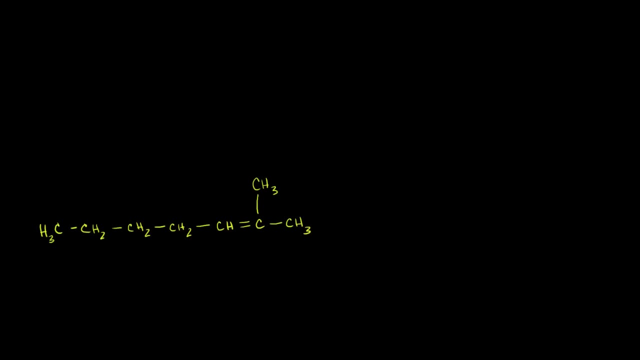 And I also have some side chains, So let's see if we can figure out how to deal with all of these things. So, first of all, what is our longest chain of carbons? So we have 1,, 2,, 3,, 4,, 5,, 6.. 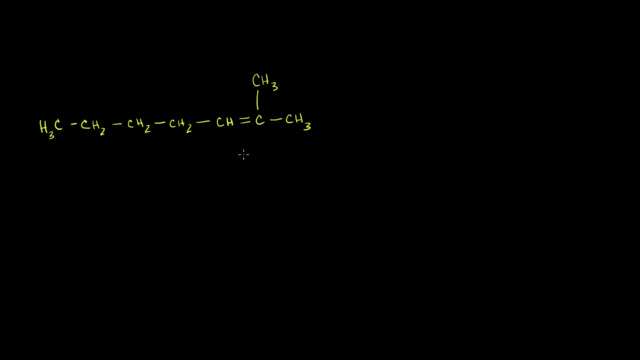 And we could go in either direction. It doesn't matter 7 carbons or 7 carbons, And let's start numbering closest to the double bond. The double bond actually will take precedence over any other groups that are attached to it. 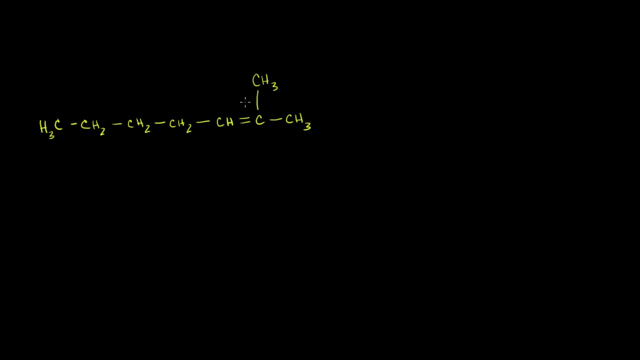 So let's take precedence over any other groups in this case. There will be other groups that will take precedence in the future, But the double bond takes precedence over this side chain, this methyl group, But it doesn't matter in this case. We'd want to start numbering at this end. 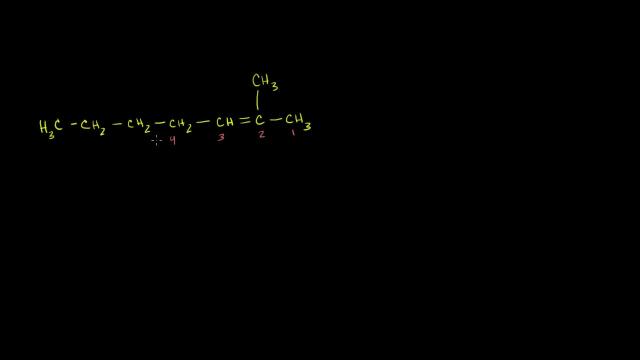 So it's 1, 2 carbon, 3 carbon, 4 carbon, 5 carbon, 6 carbon, 7 carbon. So we're dealing with a hept again. So we're dealing with a hept And we have a double bond starting from the second. 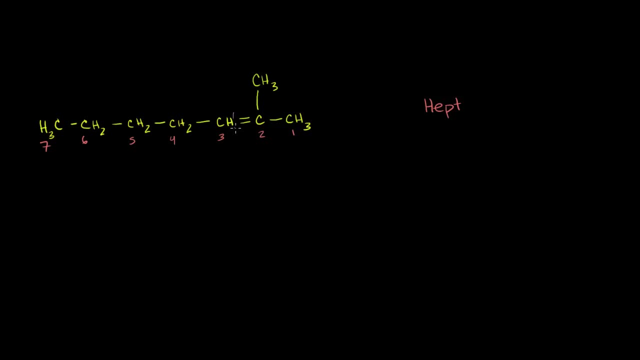 carbon to the third carbon. So this thing right here, this double bond from the second carbon to the third carbon, So it's hept, 2 comma 3, ene. Sorry, not 2 comma 3, 2-ene. 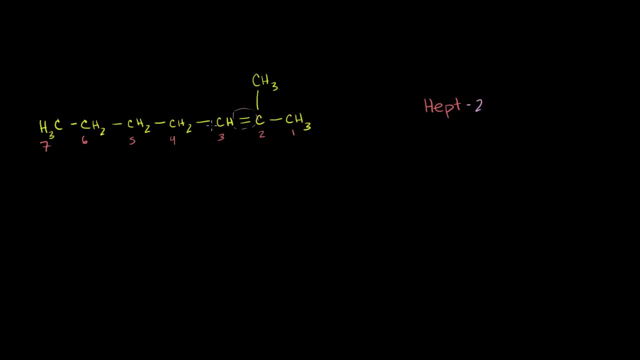 You don't write both endpoints. If there was a 3, then that would have been another double bond. there It's hept, dash, 2, dash, ene. And then we have this methyl group here which is also sitting on the second carbon. 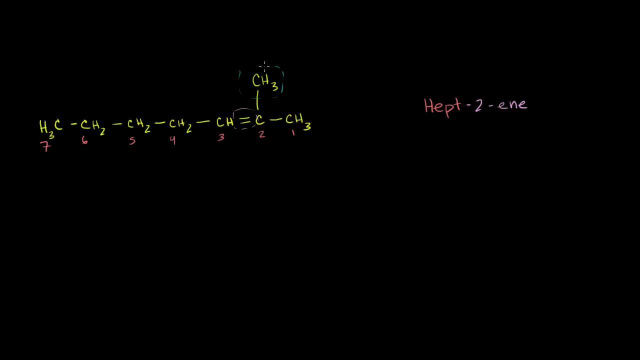 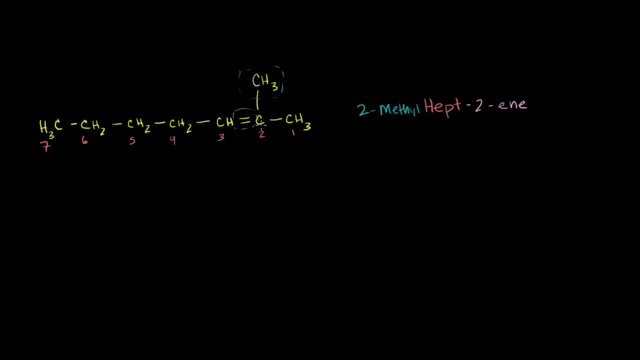 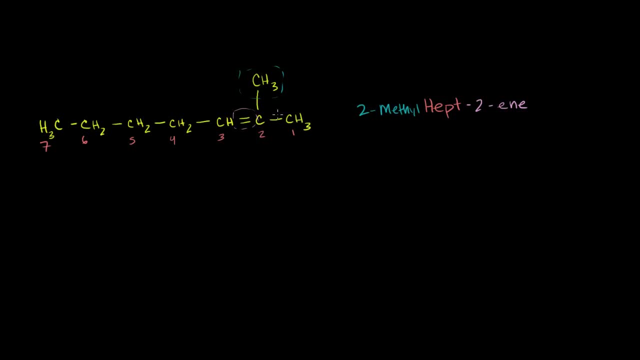 numbering from the right. And then the methyl group is also attached to that second carbon. Let's do one more of these. So we have a cycle here, And once again the root is going to be the largest chain or the largest ring here. 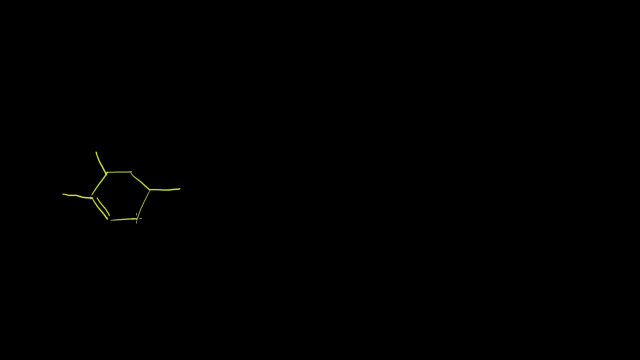 And our main ring is the largest one And we have 1,, 2,, 3,, 4,, 5, 6 carbons. So we are dealing with hex As our root for kind of the core of our structure. 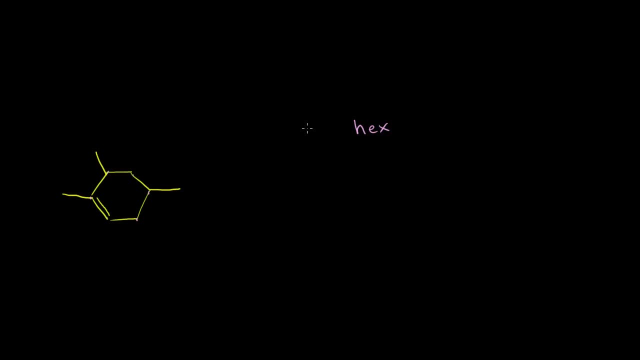 And it's in a cycle, So it's going to be cyclohex. So let me write that. So it's going to be cyclohex, But it has a double bond in it, So it's cyclohexene. Let me do this in a different color.